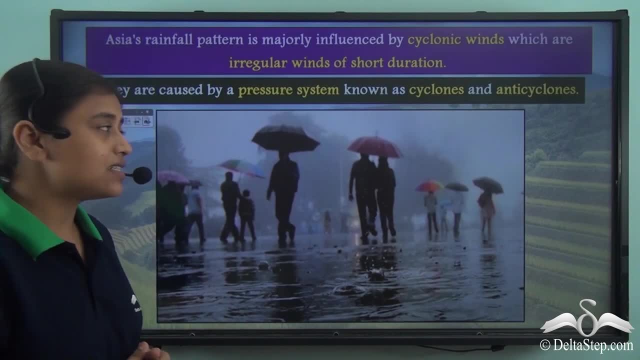 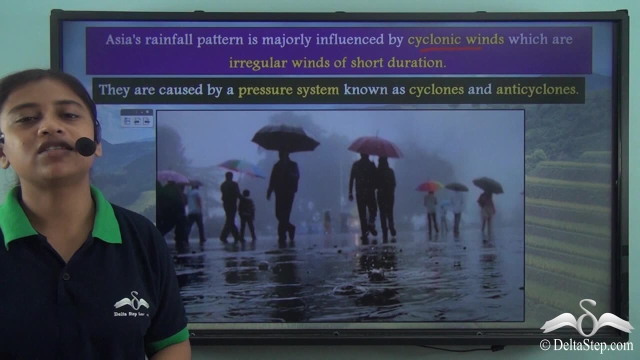 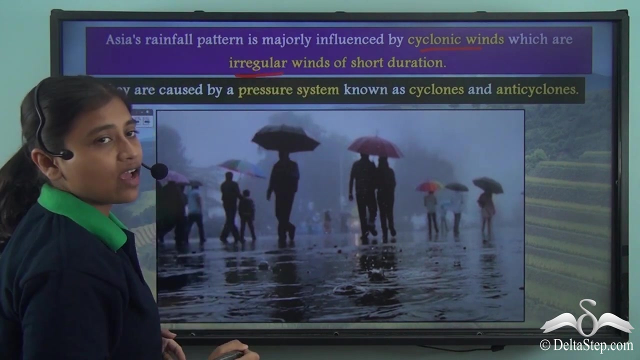 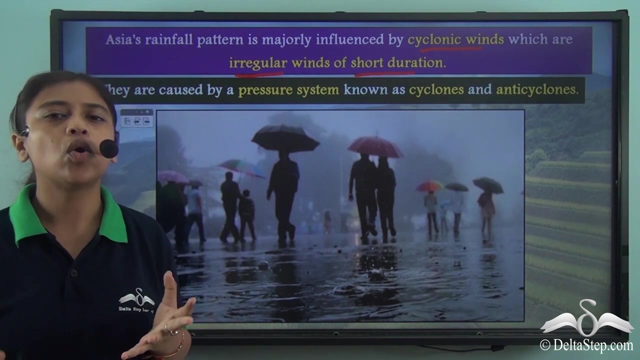 that influences the rainfall pattern of Asia is the cyclonic winds, So Asia's rainfall pattern is majorly influenced by the cyclonic winds. Now, these cyclonic winds are winds that are irregular and unstable and they are of short duration. Now, where do these cyclonic winds emerge from or originate? So they are a result of certain pressure system that exist over the continent of Asia Right. So the cyclonic winds are a result of a pressure system known as the cyclones and anticyclones. So cyclones and anticyclones are pressure systems that helps in the development of cyclonic. 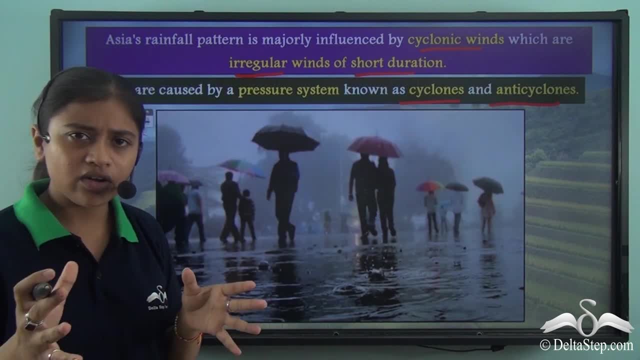 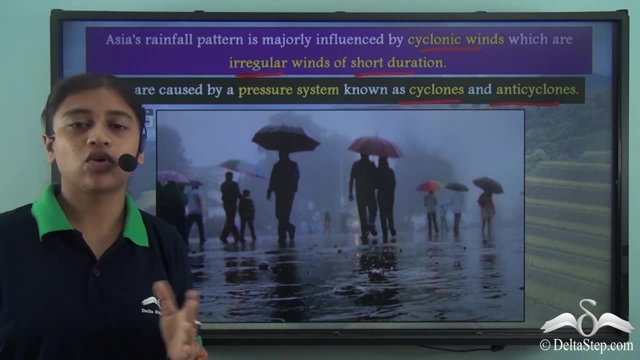 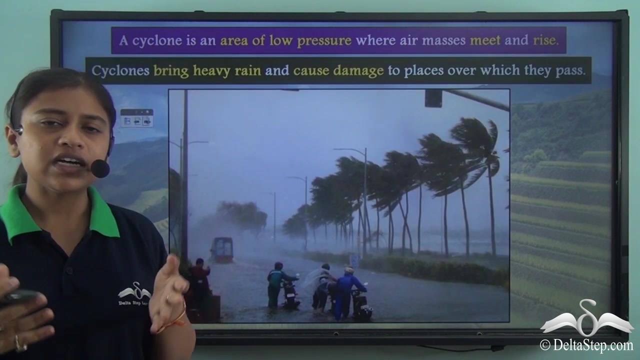 winds, and these cyclonic winds, which are irregular and of short duration, influence Asia's rainfall pattern. Now how all of this goes about is what we need to look at. So we need to first understand what exactly is a cyclone and anticyclone as a pressure. 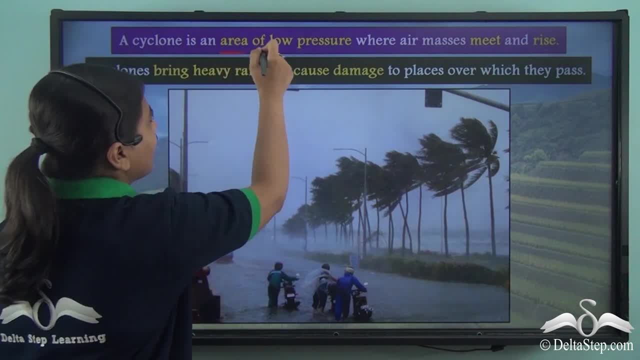 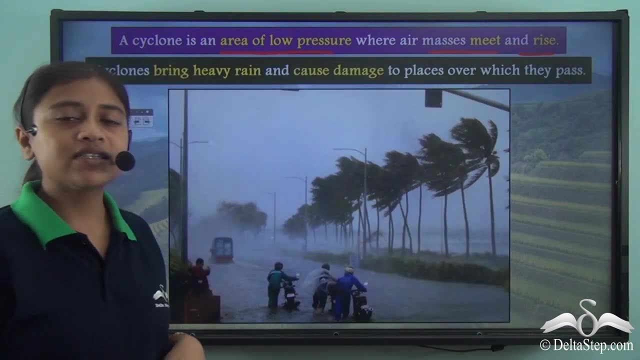 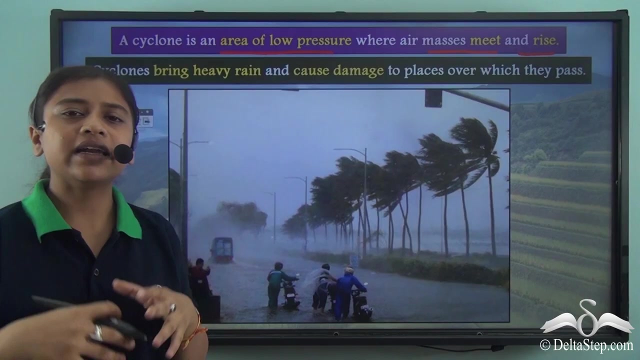 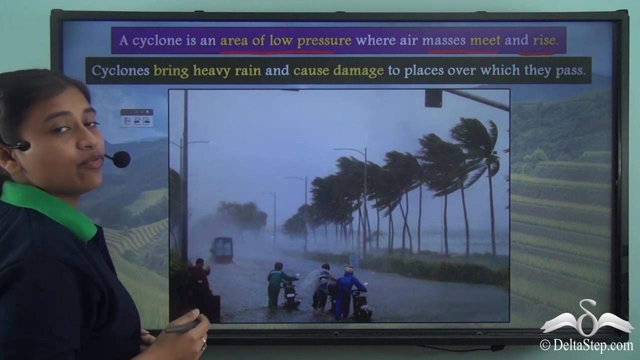 system. So cyclone is an area of low pressure where the air masses meet and rise. So it is an area of low pressure where the air comes together and then they rise. So in a cyclone or an area of low pressure where the winds meet and rise, there we have. 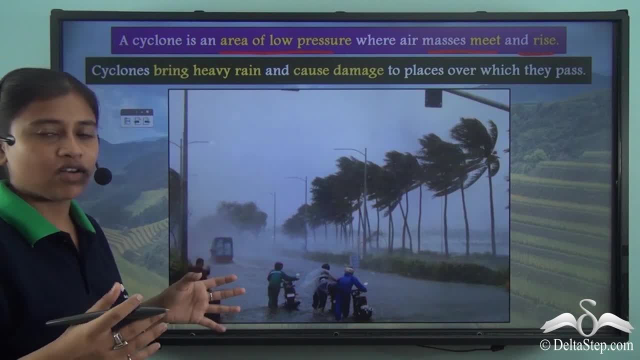 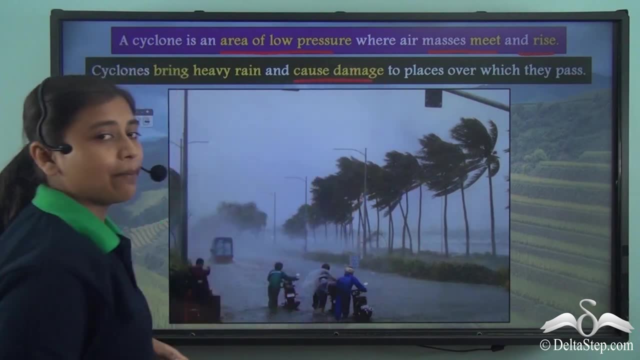 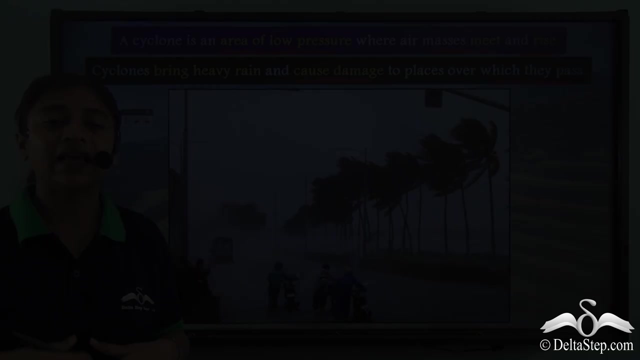 a bad weather. So we can often say that a cyclone usually indicates a bad weather, And sometimes they can also cause big damage to places over which they pass. So a cyclone usually brings along bad weather, like clouds or heavy rainfall that might sometime. 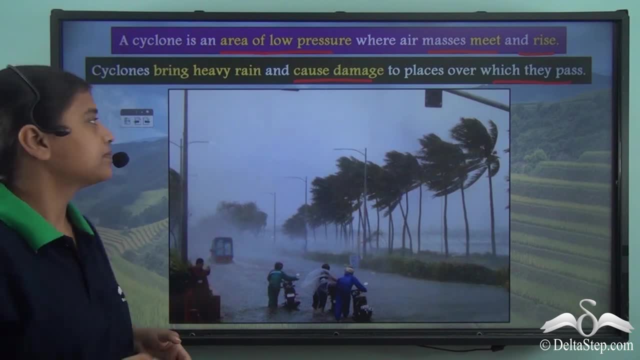 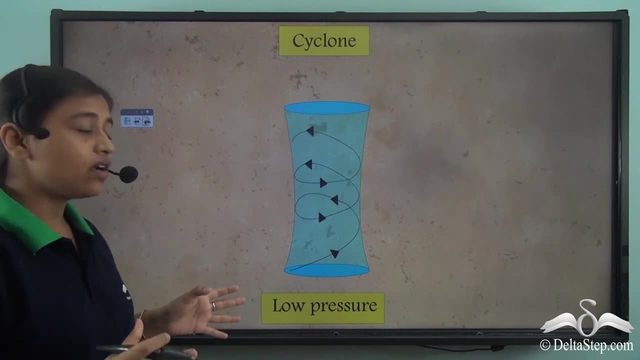 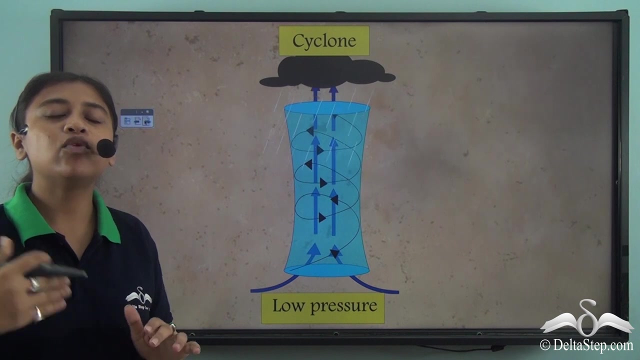 cause huge damage to places from where they pass. So let's see how a cyclone works. So cyclone is where the winds come together, that is, they meet in a low pressure, They are in a low pressure area at the surface of the earth and they move in a spiral way. 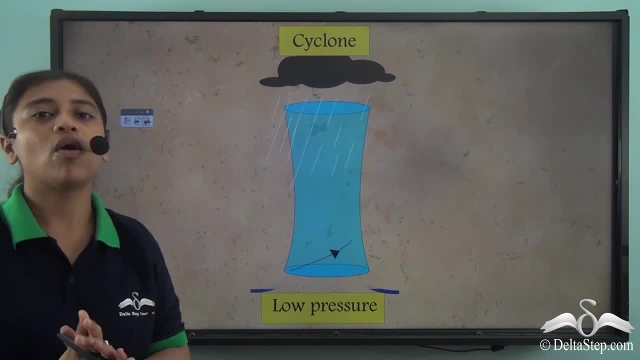 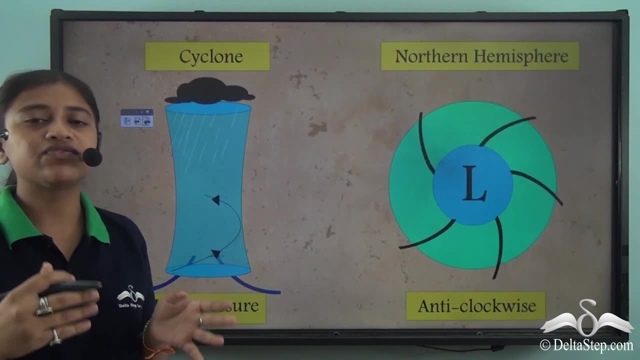 They come and they meet, and they rise up to form clouds, which then brings heavy rainfall over the places where they pass from. Now they have a different movement in the northern and southern hemisphere. In the northern hemisphere they move in an anticlockwise direction, and in the southern 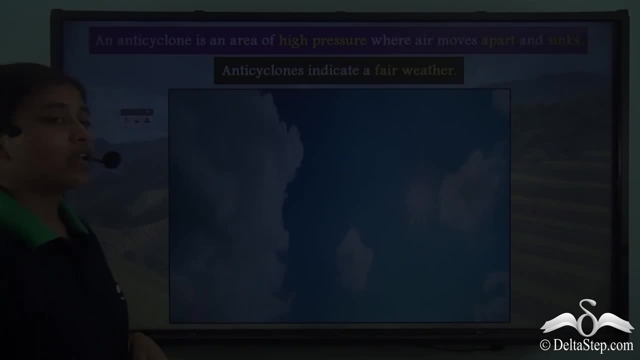 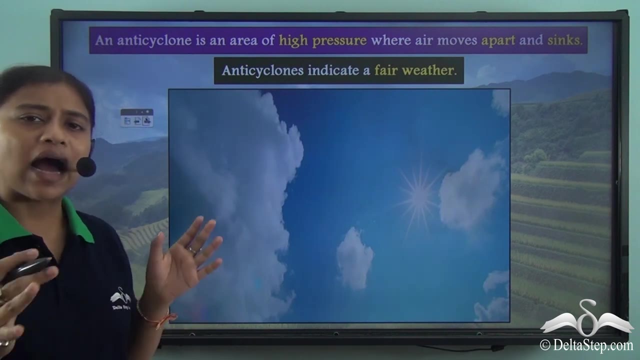 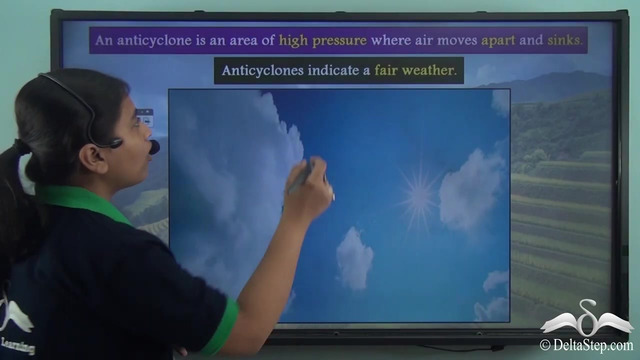 hemisphere in a clockwise direction. So that was about the cyclone. Now let us look at another pressure system and that is the anti-cyclone. So anti-cyclone is right opposite to a cyclone. In an anti-cyclone, we have an area of high pressure where the air moves apart and sinks. 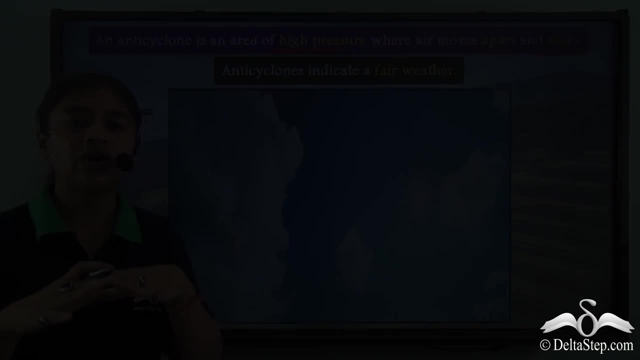 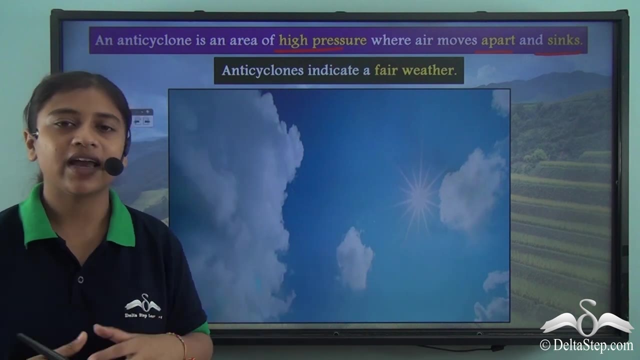 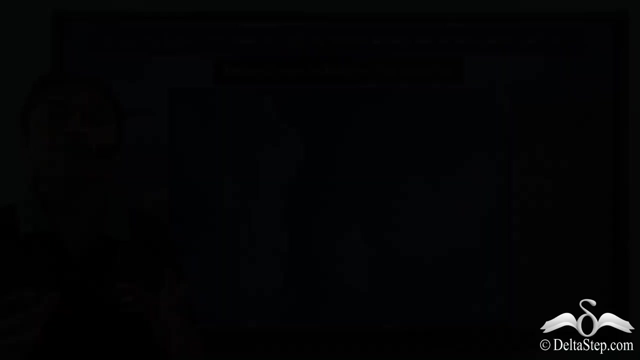 So there from the high pressure area, the winds or the air, they move apart and they sink and they move towards the low pressure area surrounds the high-pressure area. So in an anticyclone we have a high-pressure area right where the air moves apart from the center of high-pressure area. 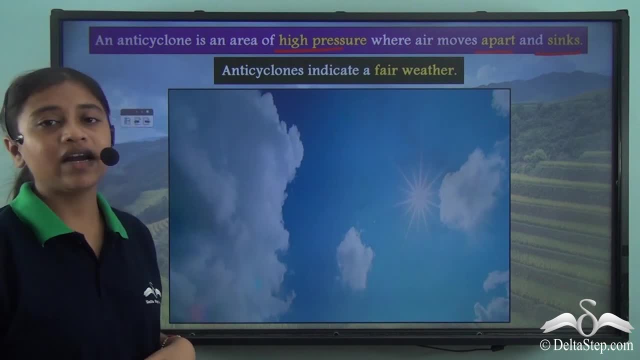 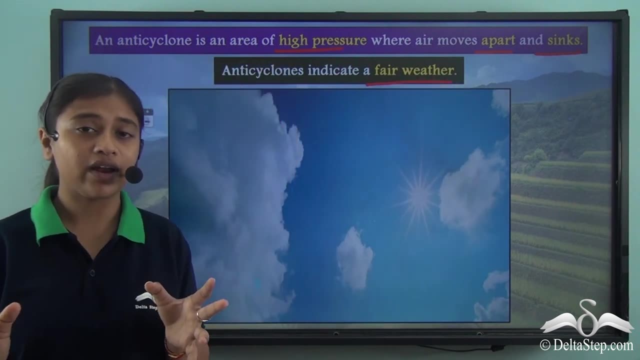 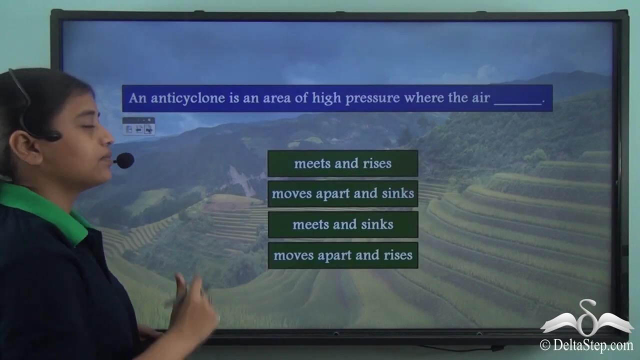 and they sink. Now, unlike the cyclone, an anticyclone indicates a fair weather. So, while a cyclone brings along heavy rainfall and can cause damage, an anticyclone is what indicates a fair weather. But before we proceed with our lesson, could you help me answer this simple question? An anticyclone is an. area of high pressure where the air meets and rises, moves apart and sinks: meets and sinks or moves apart and rises. Which will be the correct answer? Well, the correct answer is: the air in an anticyclone moves apart and sinks, So move apart from the centre of a high pressure area and they sink to go on to places that are low pressure area right. So in an anti-cyclone the air moves apart from the centre, that is, the high pressure area, and then it sinks. So opposite happens in a cyclone situation. Now, in an anti-cyclone in the northern hemisphere, the air moves apart from the high pressure. 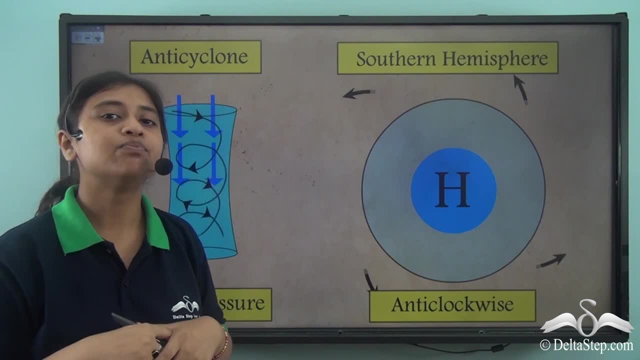 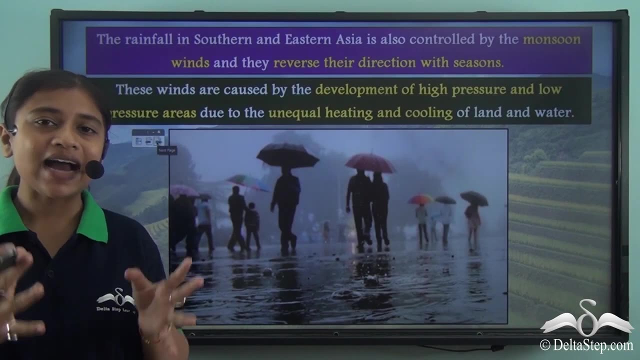 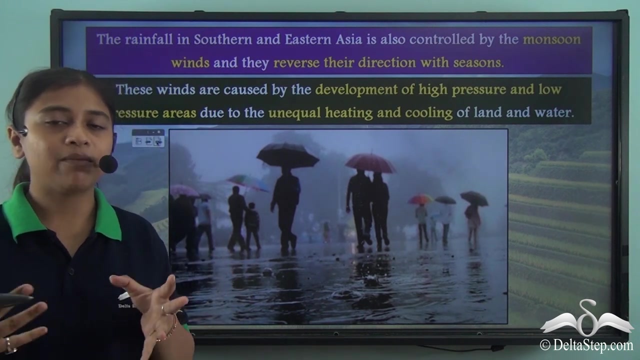 area in a clockwise direction and in the southern hemisphere is move apart in the anti-clockwise direction. So that is where we saw how anti-cyclones and cyclones, both having its own characteristics, influence the rainfall pattern of Asia. So places that are of high pressure are places 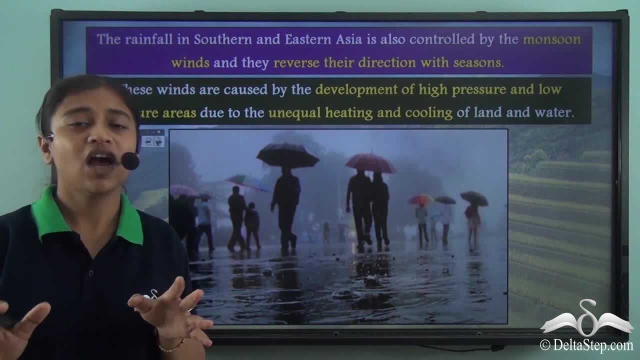 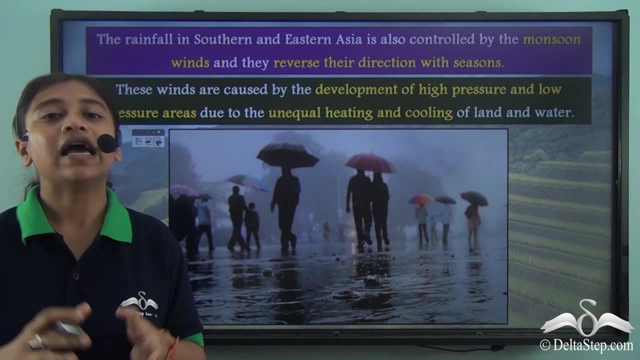 of anti-cyclone or experience of fair weather, that is, they do not experience heavy rainfall. However, places of high pressure are places of high pressure. So, in the case of high pressure, places that are of low pressure are area where the air meets and they rise, creating clouds and thus. 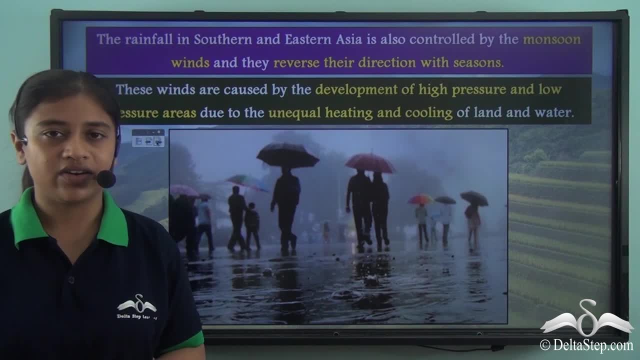 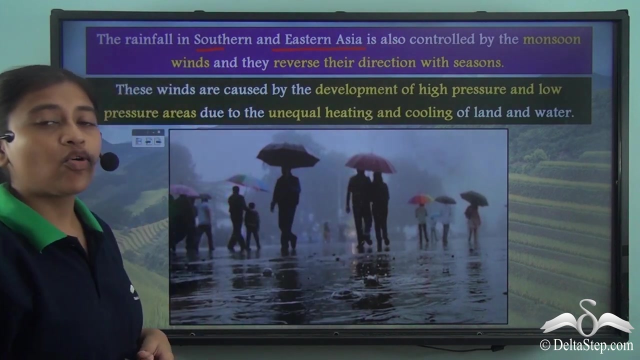 leading to heavy rainfall. So those are cyclone areas. Let's move on to look at another factor that has a huge influence on the rainfall pattern of Asia. So the rainfall in the southern and eastern part of Asia is controlled by monsoon winds, right. So they are highly influenced by 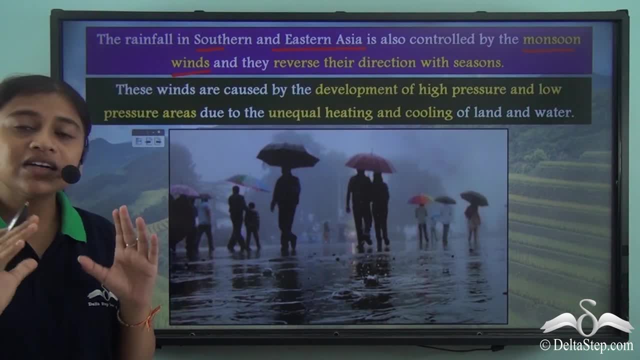 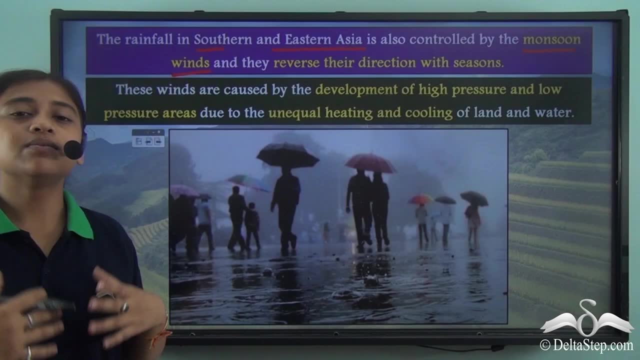 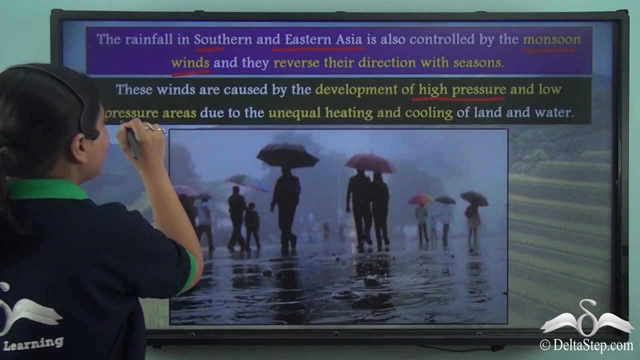 monsoon winds, and these monsoon winds reverse their direction with seasons. Now, what exactly are these monsoon winds and how do they work? So these monsoon winds are a result of, or are developed from of high pressure and low pressure areas due to unequal heating and 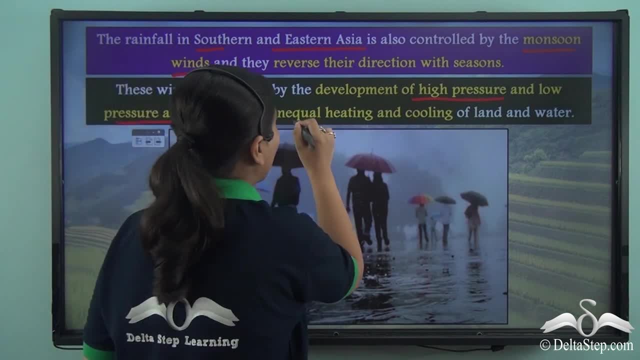 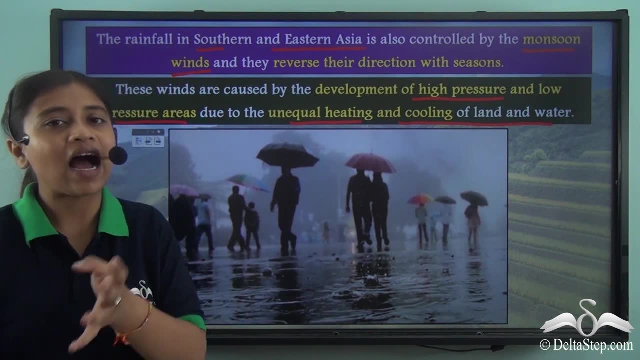 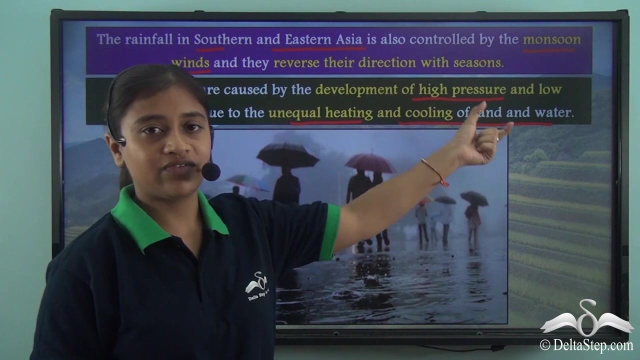 cooling of land and water right. So unequal heating and cooling of land and water leads to the creation of low pressure area and high pressure area, and that gives rise to monsoon winds. We will look at each of these factors that leads to the development of monsoon winds. 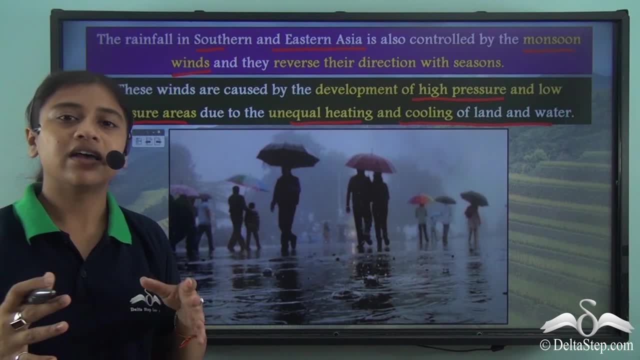 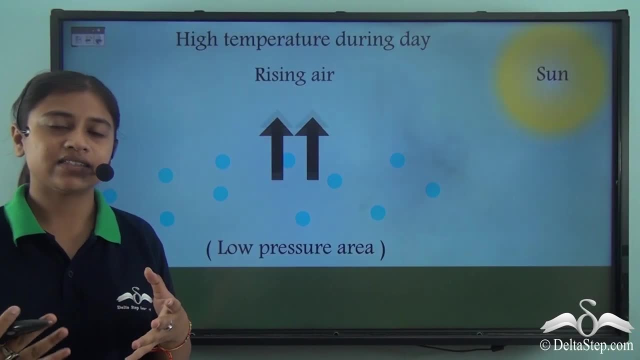 and then understand how these monsoon winds influence the rainfall pattern of Asia. So during daytime, we know that lands get heated up faster, So there's high temperature during daytime. There the air becomes light, There the air becomes light, becomes light and it rises, creating a low pressure area. However, during night time, a opposite happens. So during night time, when the temperatures are low, there a high pressure area is created because the air becomes heavier and dense and they come together and sink. So what happens? that during day time, when the temperature is high, the air rises, creating low pressure area, and during night time, when the temperature is low, a high pressure area. 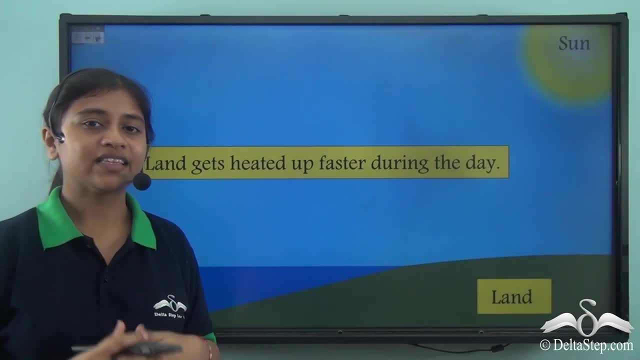 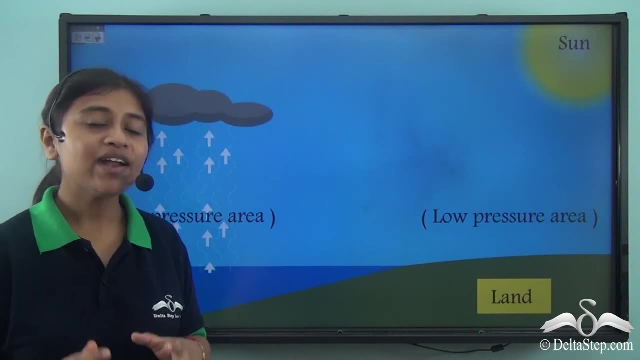 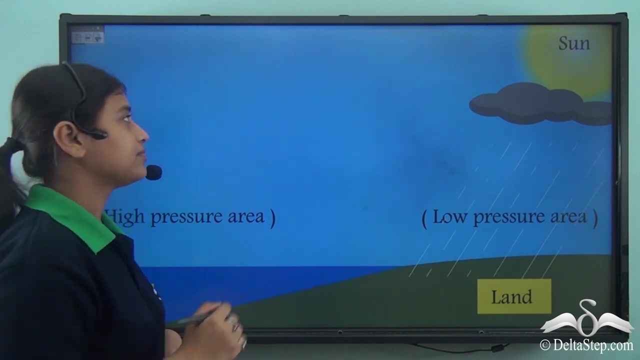 is created. So by that logic, the land gets heated up faster during the day as compared to the sea. So high pressure exists over the sea. So when air moves from a high pressure area, that is, the sea, to the land, it carries moisture and brings rainfall on the land. 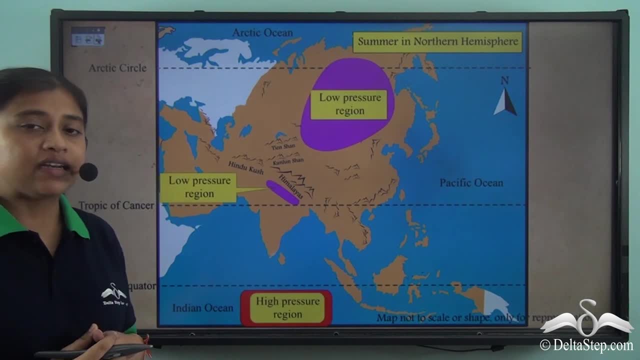 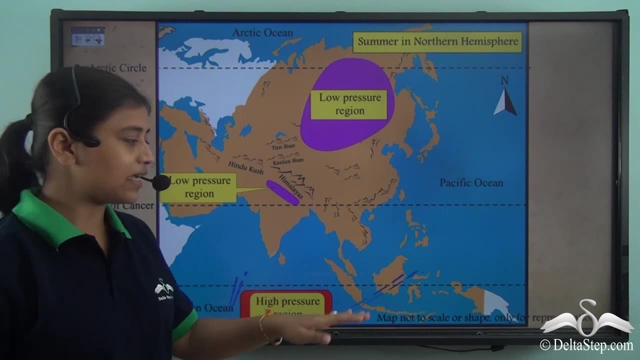 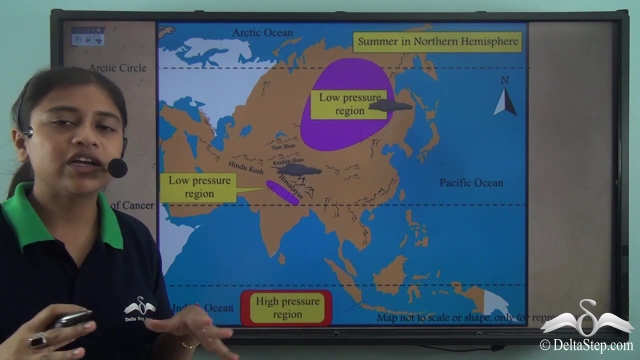 So we just understood how monsoon winds are formed or developed. Now in Asia, during April to September, that is, during the summer season, winds blow from Indian Ocean and Pacific Ocean and, due to unequal heating of land and water, a low pressure area is created over much of 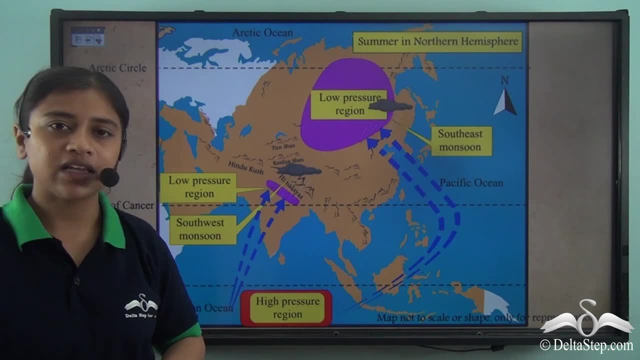 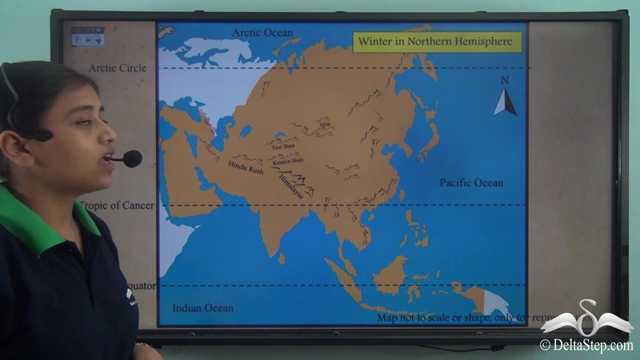 the Asian continent and a high pressure area is over the sea. These winds bring along moisture and bring rainfall in the parts where low pressure region has been created. These are south west and south east monsoon winds. Now, during winter season, a similar thing happens, but in a opposite way. So a low pressure. 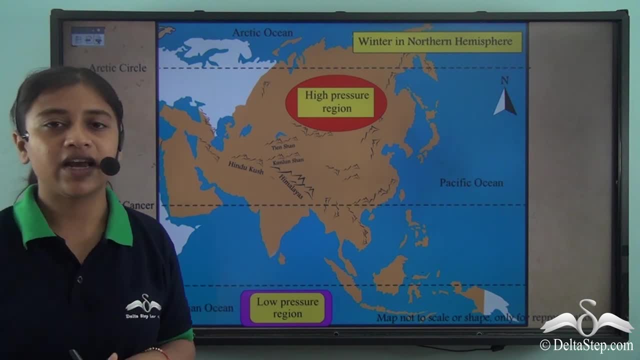 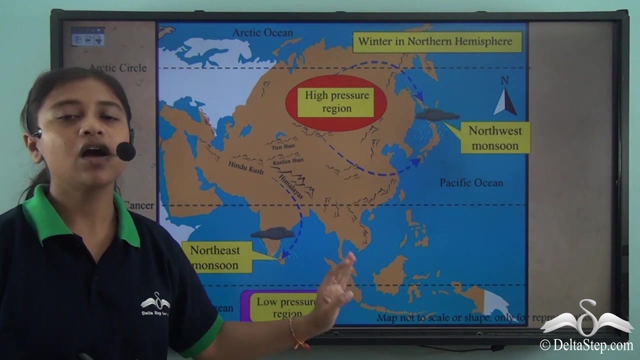 area is created over the seas and a high pressure area prevails over the land because during winter season the lands get cooler, faster than the sea. Therefore, the winds blow from the land to the sea and they bring rainfall in certain parts of Asia, mostly towards the 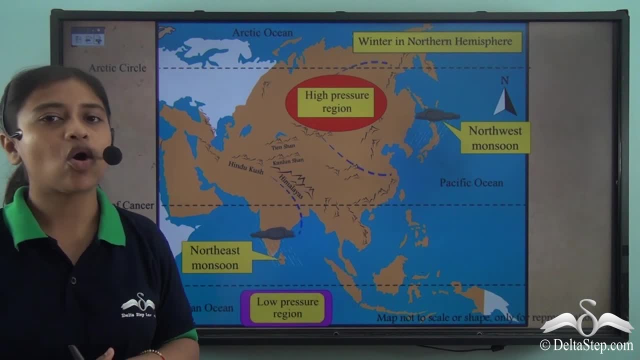 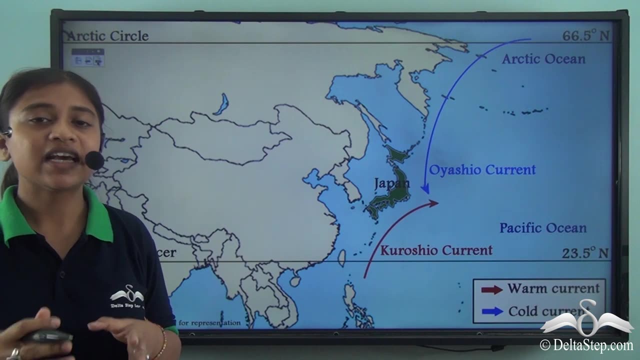 south and south eastern parts. These are the north, west and north east monsoon winds. So we just took a look at how monsoon winds influence the rainfall pattern of the Asian continent. However, ocean currents interestingly also play a very important role in influencing 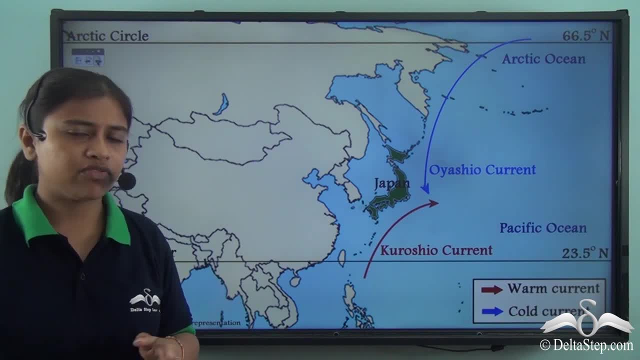 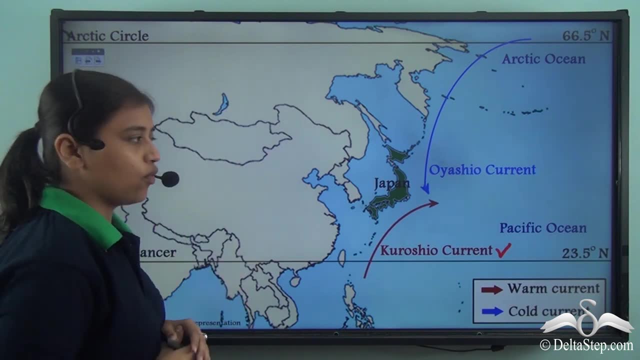 the rainfall pattern of Asia. So a very good example of the same is here. So Corotio current is a warm current. So a very good example of the same is here. So Corotio current is a warm current current, while Oashio current is a cold current. Now these warm and cold ocean currents have 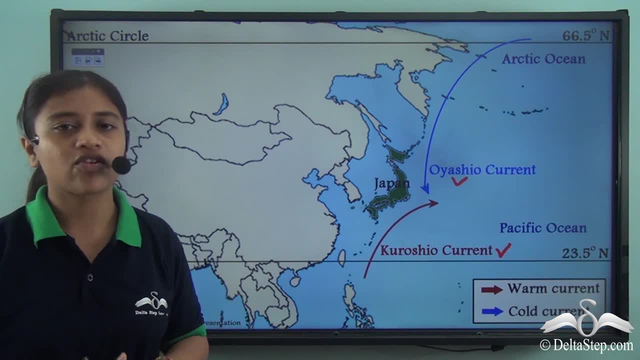 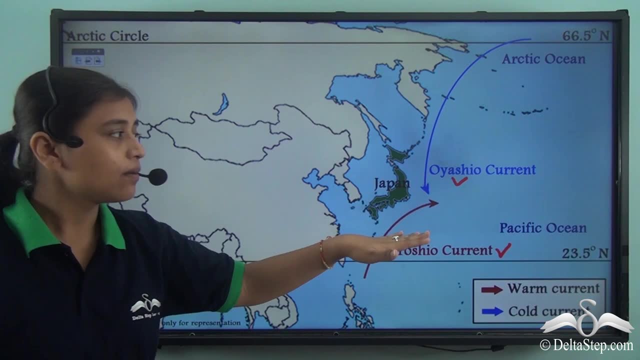 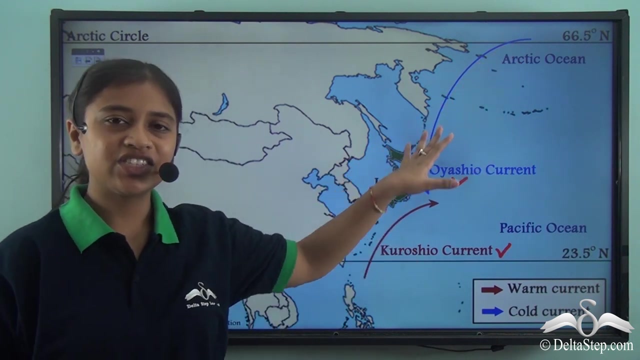 their respective influence over the areas they cross. So while Kuroshio current has a warming effect over the eastern coast of Japan, the Oashio current has a cooling effect on the same. So the Oashio current that blows from the arctic region towards or along the 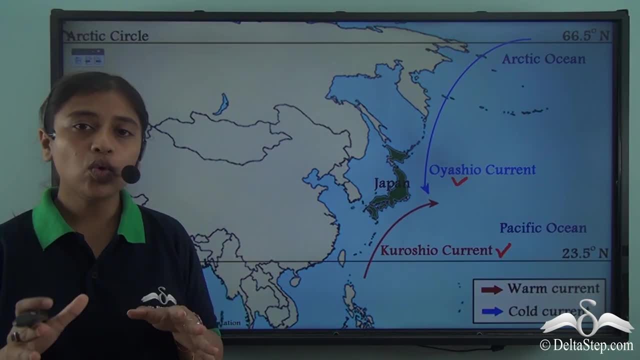 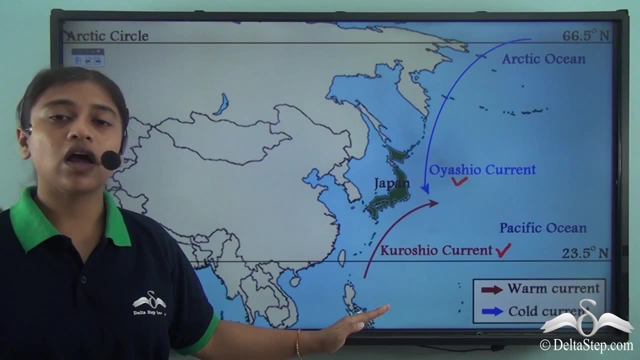 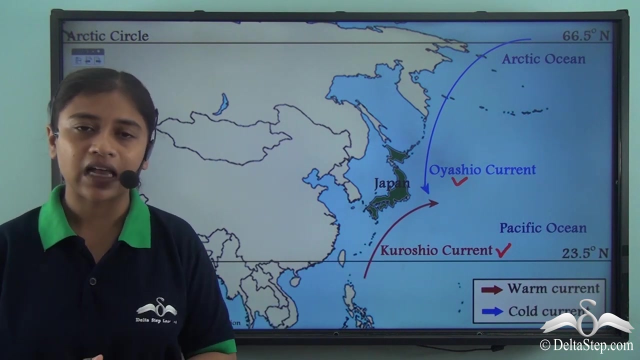 north eastern coast of Japan keeps the place cool and gives it severe winters. However, the Kuroshio current that blows from the temperate zone along the south eastern coast of Japan gives it warm summers and keeps the water here from freezing. Thus it helps in carrying 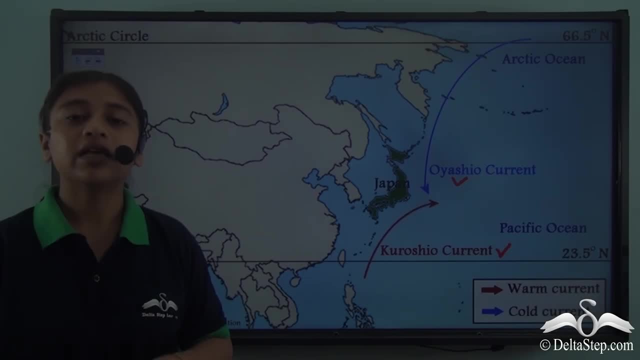 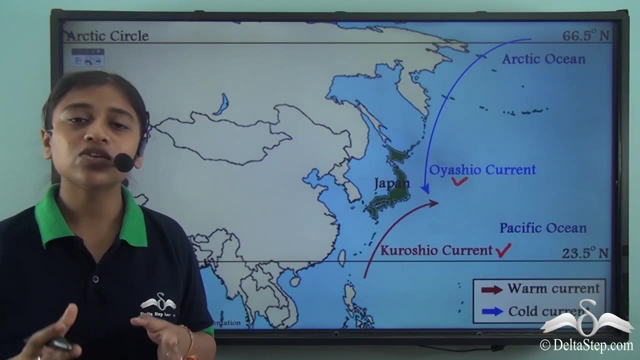 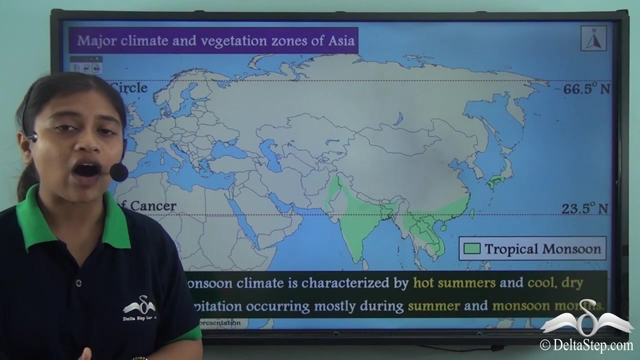 on with navigation and trade and commerce, So they both have their respective influence on the climate of Japan, And a similar thing happens to all the places or countries that are present in the coastal regions of any continent, and they are also influenced by such ocean currents. So there we got a complete insight of how. 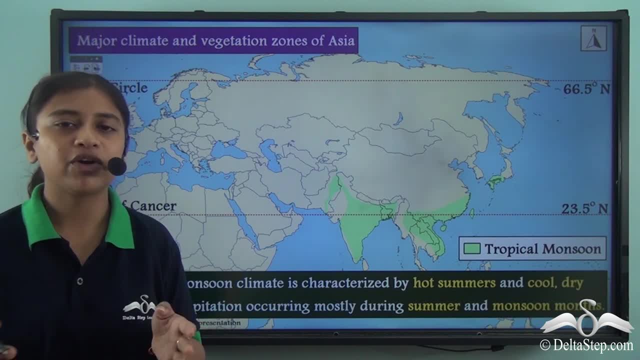 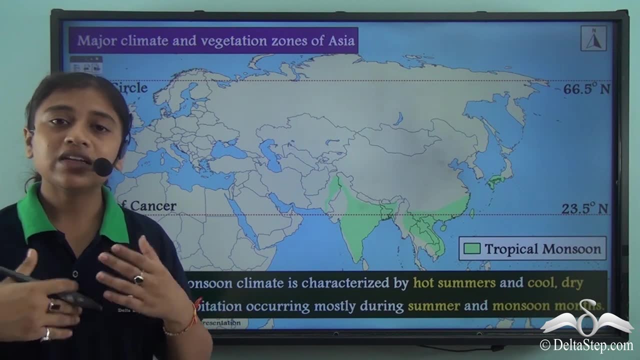 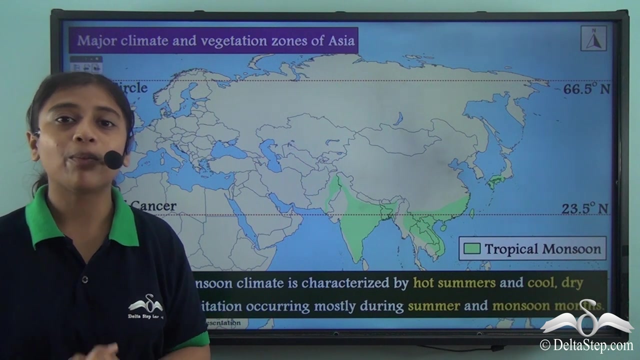 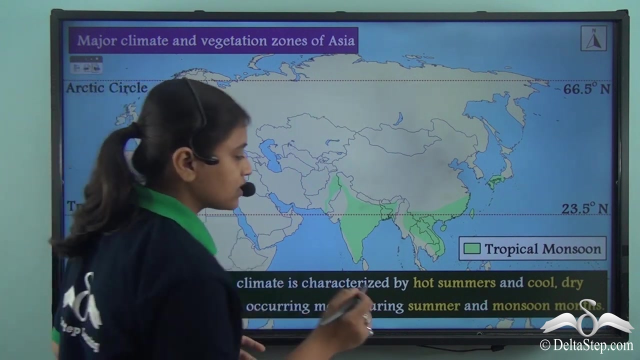 Asia's rainfall pattern is influenced by a number of factors, including the cyclonic winds, the monsoon winds and also the ocean currents. So now we can carry on with the discussion Asia by jumping into the tropical monsoon type of climate. Now, the tropical monsoon type of climate is characterized by hot summers and cool, dry. 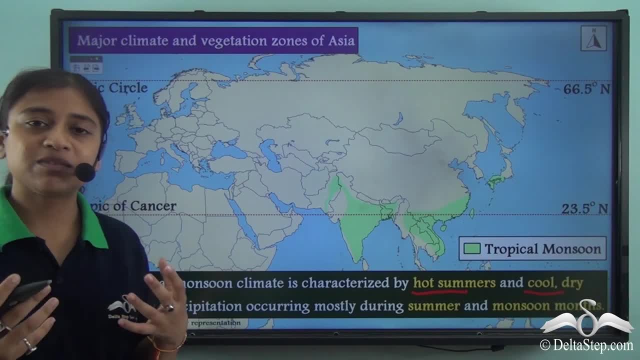 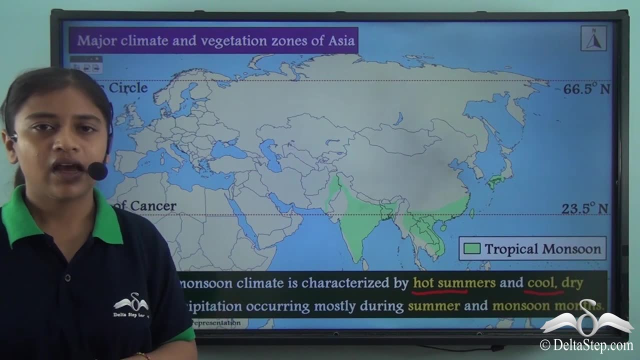 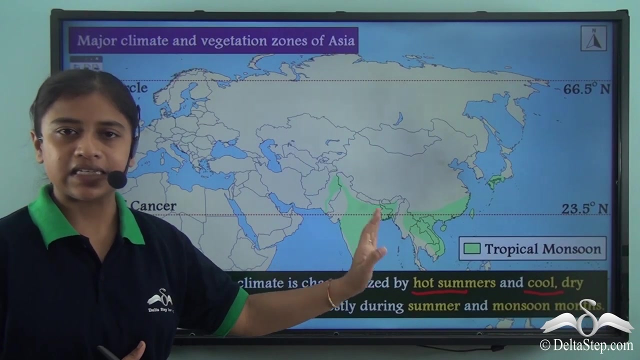 winters, And the regions that experiences tropical monsoon type of climate usually receive precipitation in the monsoon and summer months. Now we can see from the map that tropical monsoon type of climate is experienced in most parts of India and southeastern part of the continent of Asia. 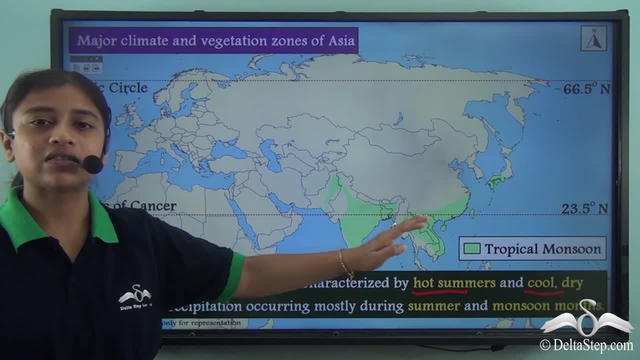 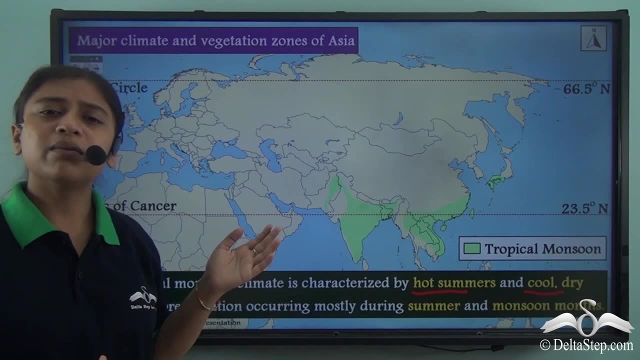 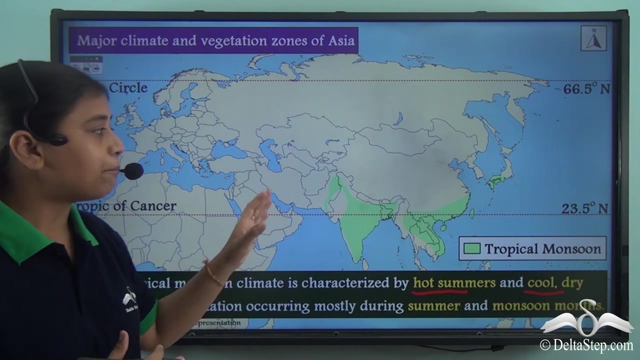 The tropical monsoon type of climate brings heavy rainfall in the southern parts of the continent, and they are characterized by hot summers while cool and dry winters. So from the map it is quite evident that the tropical monsoon type of climate mostly prevails over regions that include parts of Pakistan, India, Bangladesh, Myanmar, southeastern China. 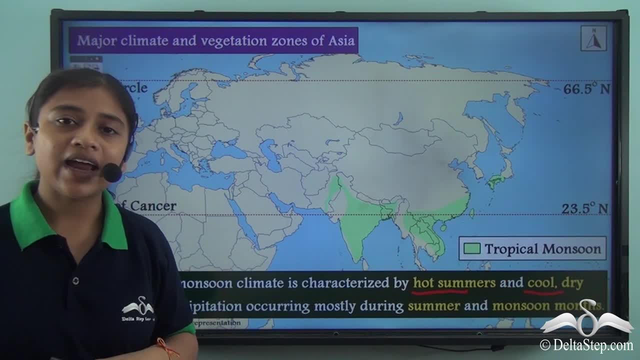 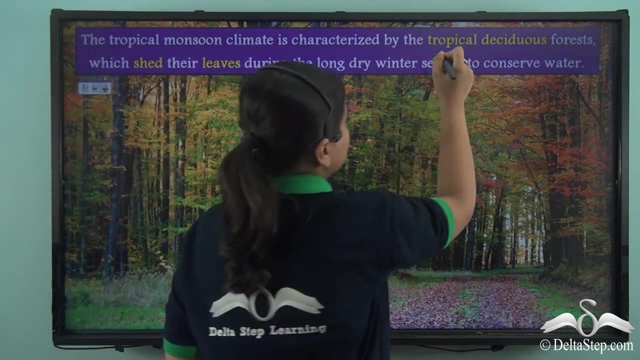 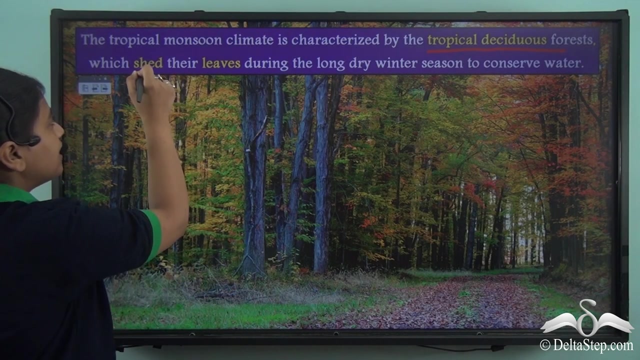 and also parts of Japan. So there they bring heavy rainfall during summer and monsoon months, and they also give them hot summer and cool, dry winters. Now, such a climate is also characterized by tropical deciduous forest, and the trees of these tropical deciduous forests shed their leaves during long dry winter season to conserve. 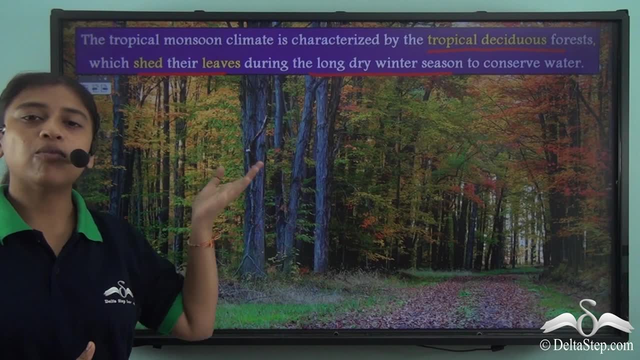 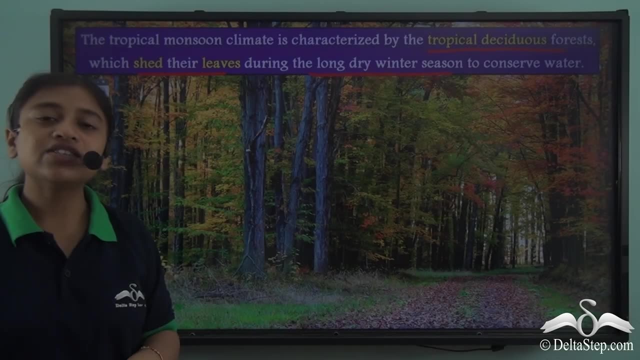 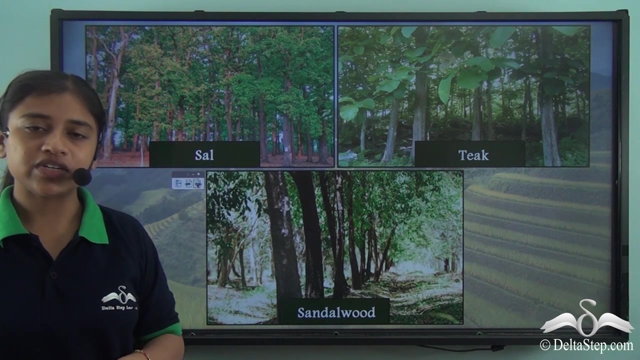 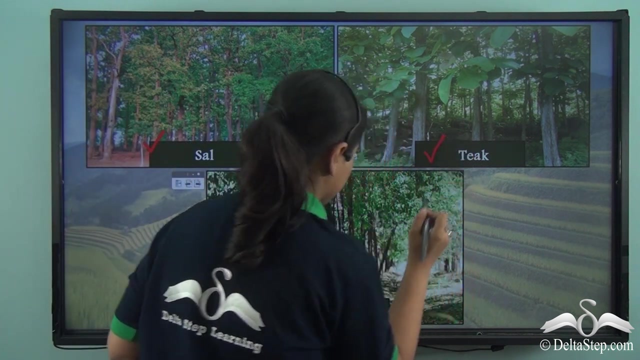 water. So the tropical monsoon type of climate usually gives rise to, or is characterized by, tropical deciduous forest trees, of which shed their leaves during long dry winters. Some important trees as part of tropical deciduous forest are saal, teak and sandalwood. 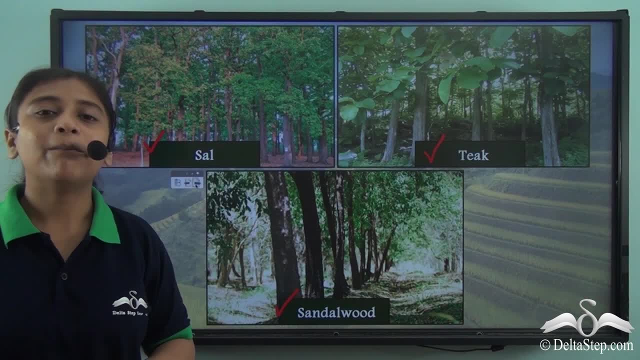 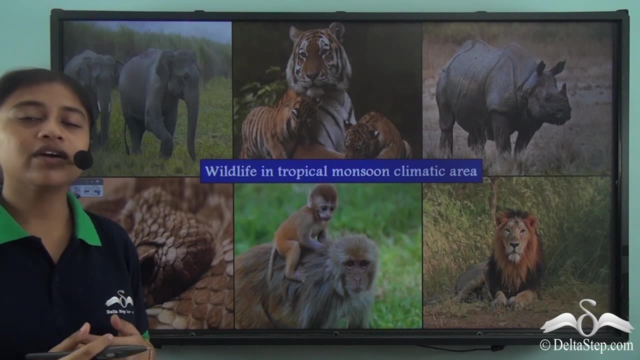 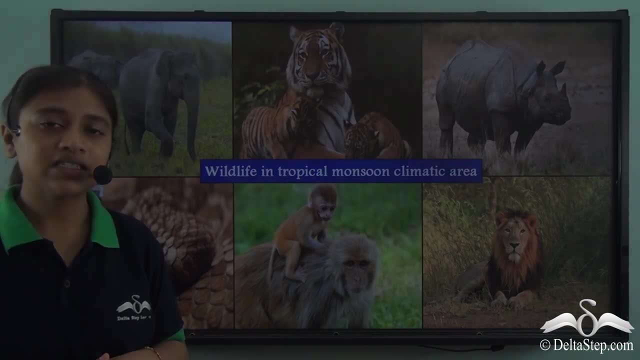 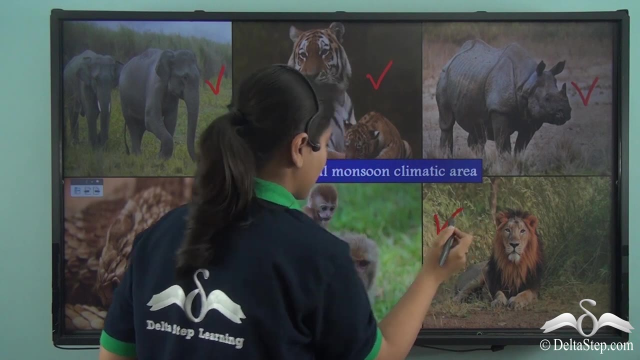 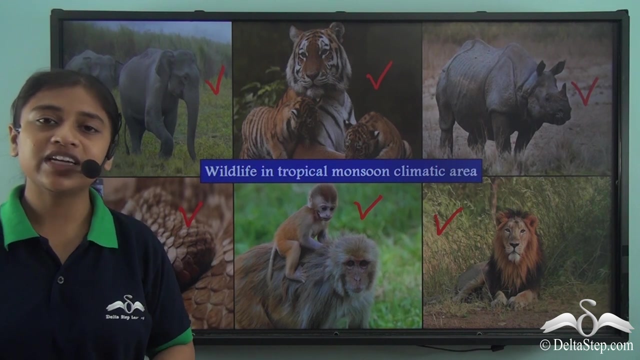 So the regions that experience tropical monsoon climate have elephants, tigers, rhinosaurus, Asiatic lion, monkeys and also snakes, So these are most commonly found animals in regions like Pakistan, India, Bangladesh, India, Pakistan, India. So these are most commonly found animals in regions experiencing tropical monsoon climate. 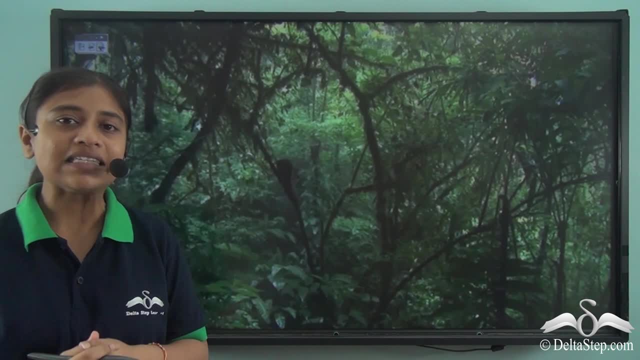 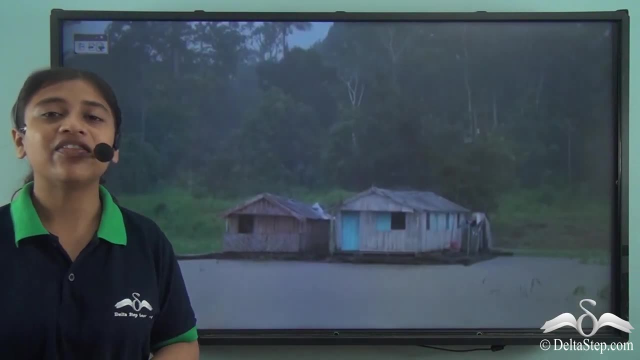 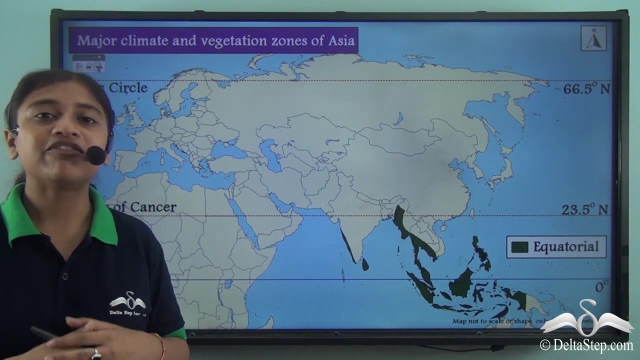 The tropical evergreen forests are characterized by high temperatures and abundant amount of rainfall throughout the year. The trees here, as you can see, are evergreen and they are beautiful. Now such tropical evergreen forests can be found in regions experiencing another major climate type that prevails in the continental climate. 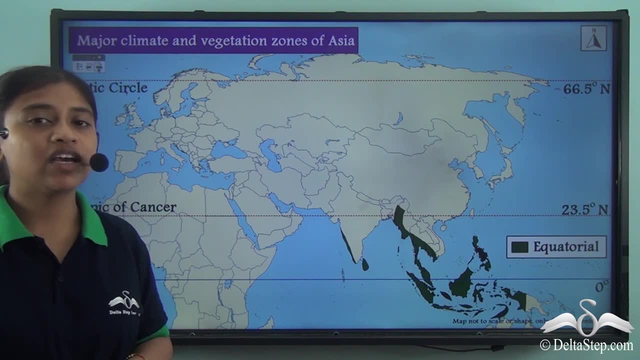 So these are most commonly found animals in regions experiencing tropical monsoon climate. The tropical evergreen forests can be found in regions experiencing tropical monsoon climate. The tropical evergreen forests can be found in regions experiencing tropical monsoon climate, And here we are referring to the equatorial type of climate. 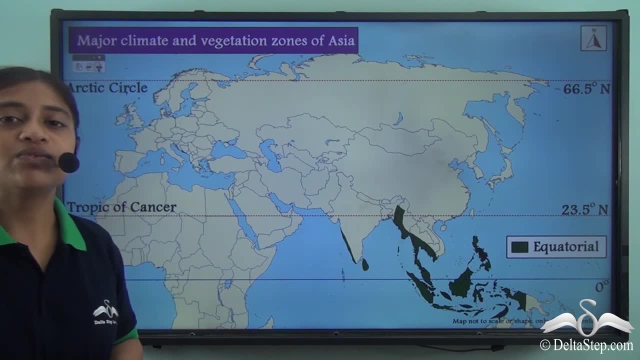 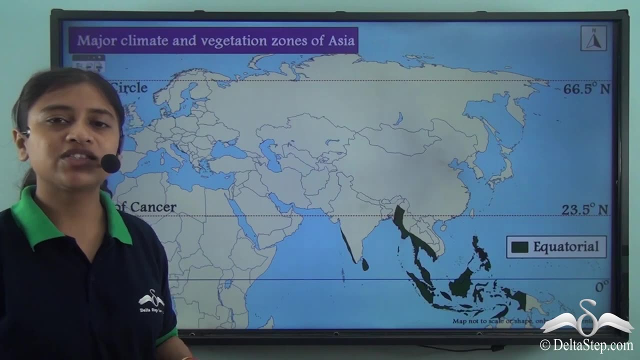 Now, the equatorial type of climate, as you can see in the map, is mostly prevalent in areas including the Indonesia and Philippine archipelagos, and also parts of India and Sri Lanka. So these areas are places that have a huge influence of the equatorial type of climate. 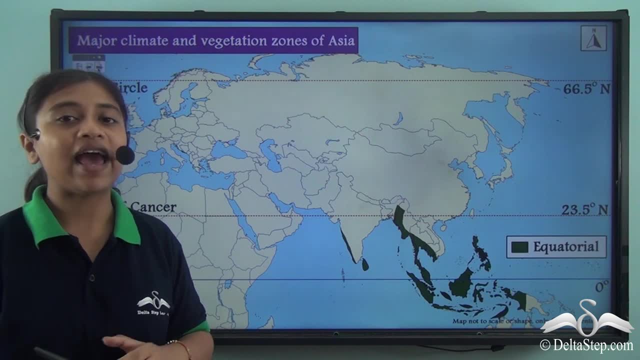 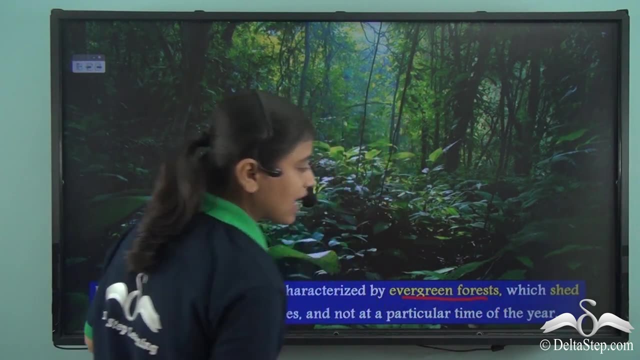 and also are places where we could find those beautiful evergreen forests, are places The tropical evergreen forests are mostly prevalent in the continental climate because of their climate. So the equatorial type of climate is characterized by evergreen forest, as I mentioned a while. 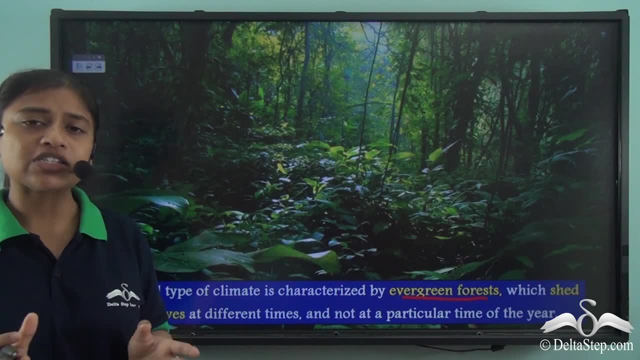 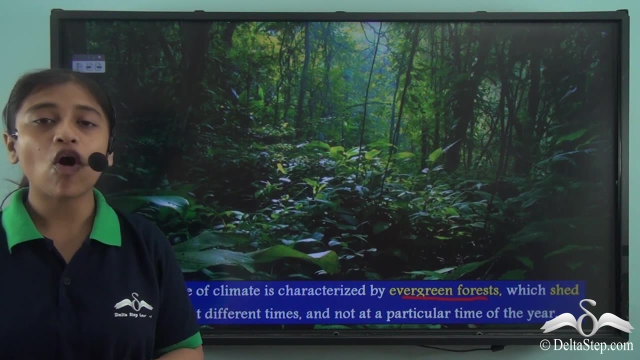 ago, and they do not shed their leaves in any one particular time of the year. So the tall trees of the evergreen forest form a canopy of leaves, that is, they form like a shelter, and there are places or the earth of these evergreen forest are believed. 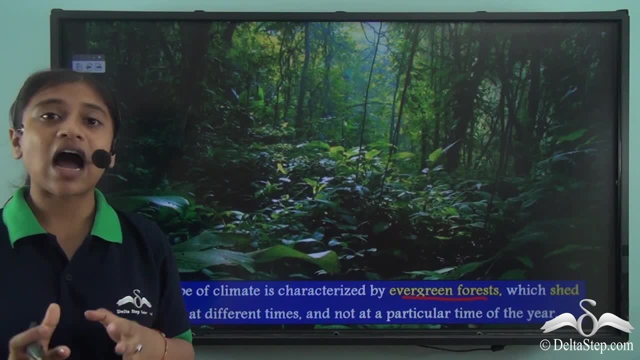 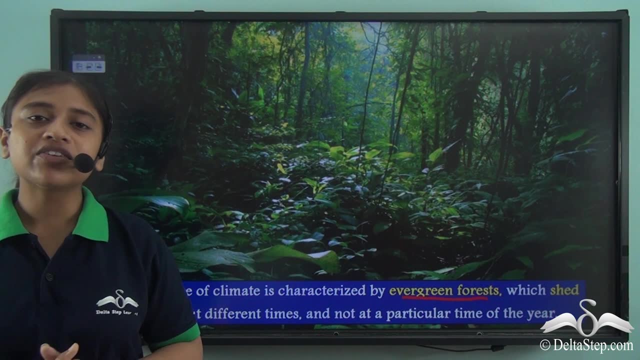 to not even receive the direct rays of the sun. This is how dense and evergreen the forest of the equatorial type regions are Now. the tropical evergreen forest have unique flora and fauna with thousands of species, some of which can only be found in these forests. 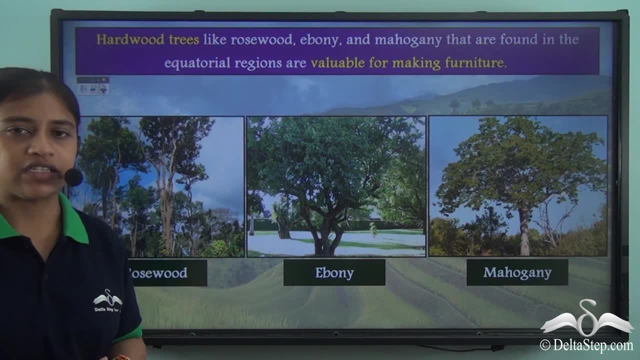 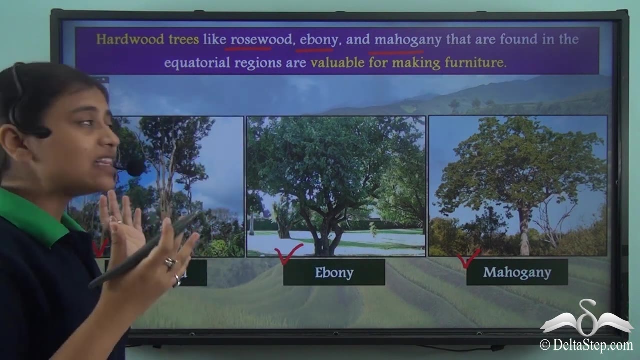 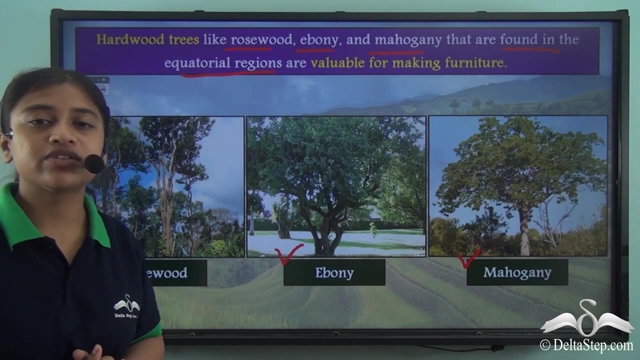 Now, the trees of these evergreen forest are hardwood trees, So hardwood trees like rosewood, ebony and mahogany, So we have pictures of all of these. So these beautiful hardwood trees that are part of the evergreen forest, and these trees are found in the equatorial regions as they are influenced by the equatorial type of climate. 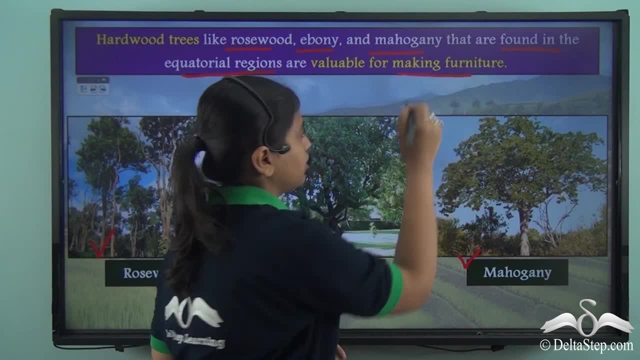 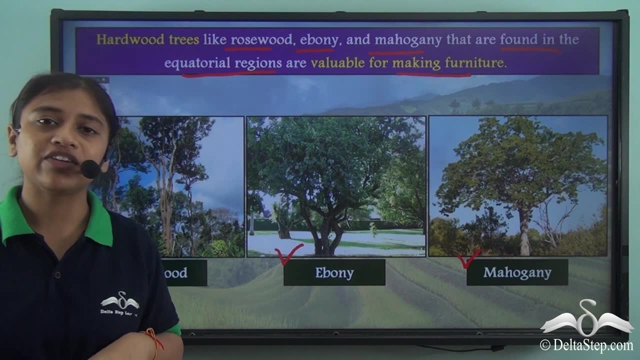 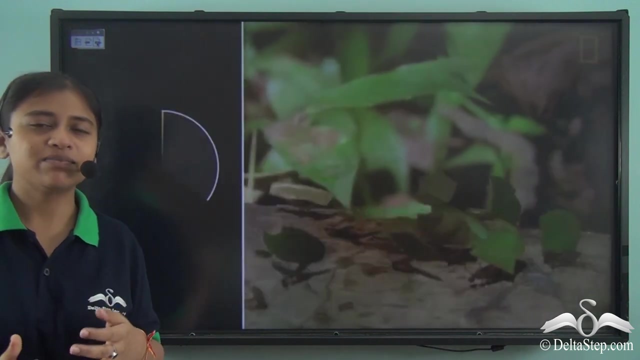 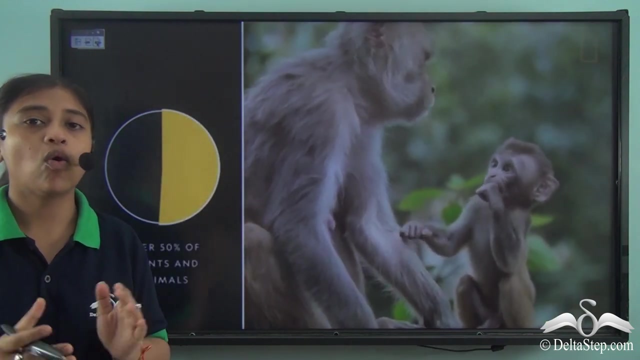 and they are valuable for making furniture. So these hardwood trees are commercially valuable and they also help in enhancing the beauty of these evergreen forests be characterized by high temperatures and abundant amount of rainfall. They are believed to cover 6% of the earth's land and are home to 50% of the animals that live on the earth. 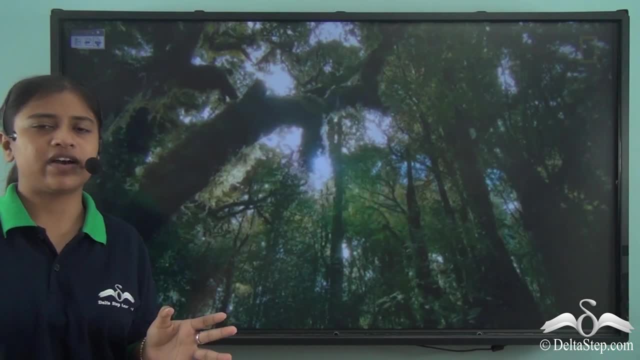 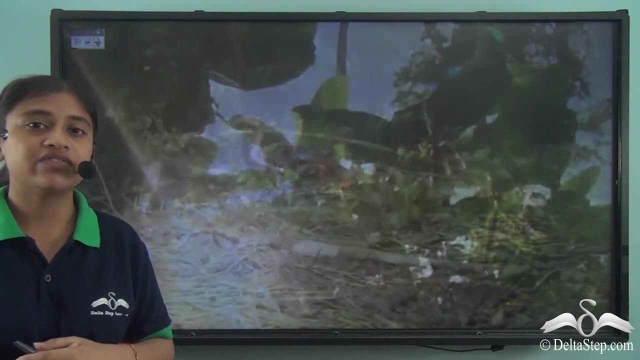 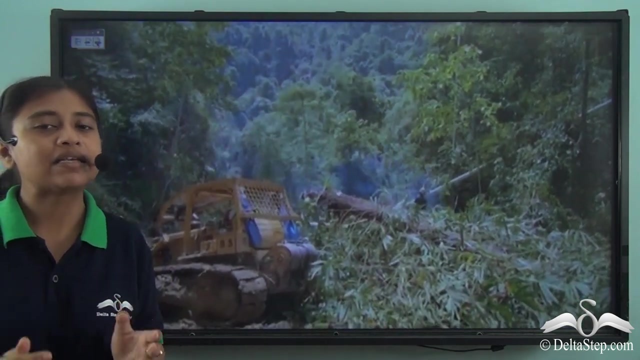 So they actually are home to unique and diversified flora and fauna. The trees here, as I mentioned ago, provide us with hardwood trees that are commercially very valuable. They also increase the beauty of these evergreen forest and a lot of which are also used for medicinal purposes. 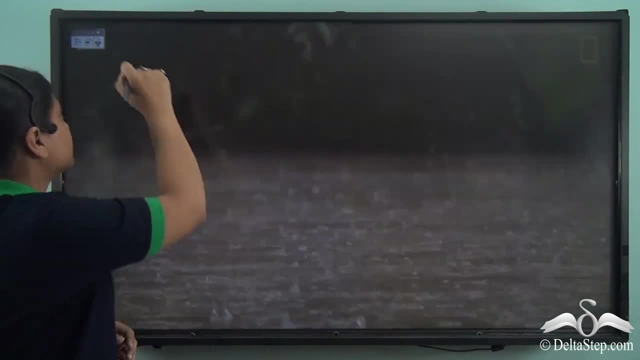 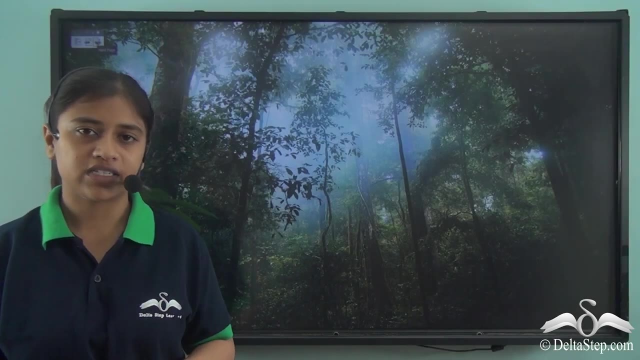 So these definitely are one of its kind. Unfortunately, due to human greed and overuse, and along with continuous deforestation, we are losing on this natural gift, So we need to be careful and find better alternative to conserve these evergreen forest. In this lesson, we were 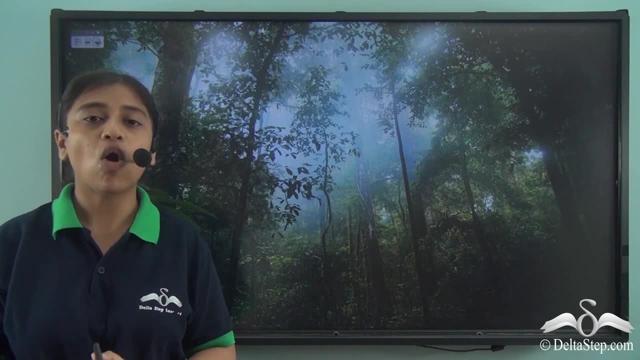 able to understand two other main reasons for deforestation. The first reason is that deforestation is not a natural phenomenon. The second reason is that deforestation is one of the major climate types of Asia and we also understood their respective vegetation and wildlife. We understood that Asia's rainfall pattern is influenced by a number 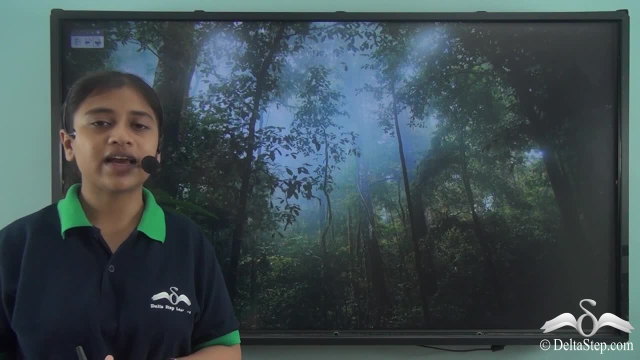 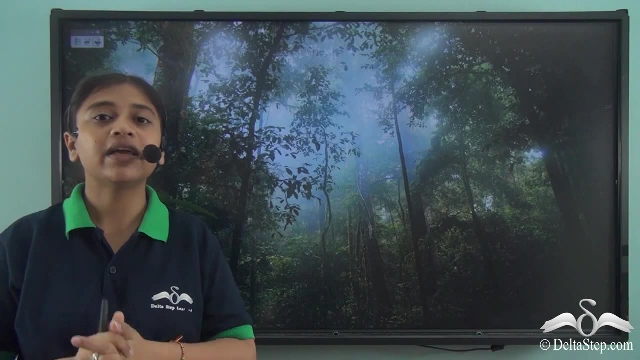 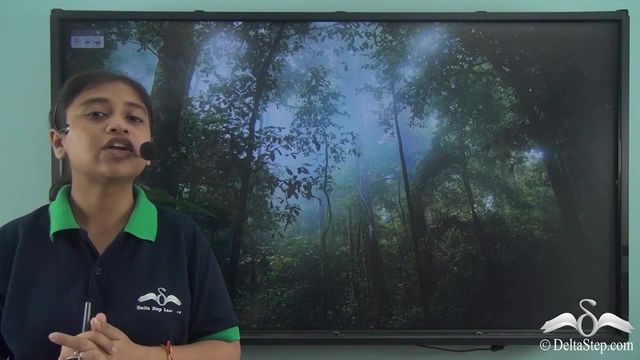 of factors like cyclonic winds, monsoon winds and also ocean currents. We further understood that the equatorial region has evergreen forests that are very important not only for the regions on which they exist, but also for people across the globe. So here we were able to conclude. 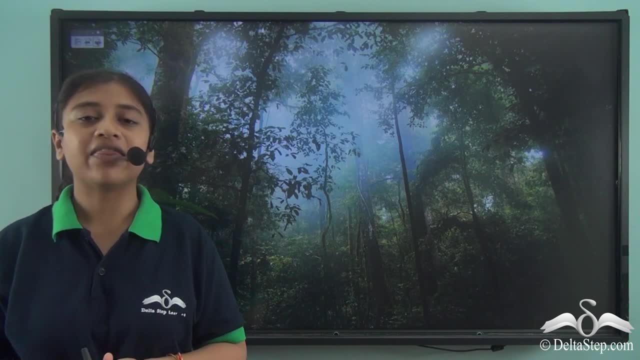 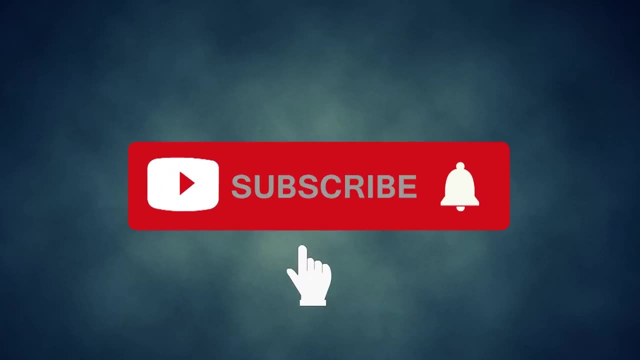 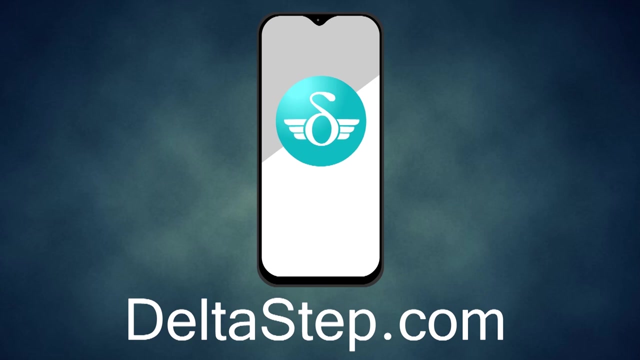 our discussion on the major climate types of Asia and their corresponding vegetation and wildlife. Don't forget to subscribe to our channel and hit the bell icon. You can also register for free at Deltastepcom or download the Deltastep app to learn one to one with our 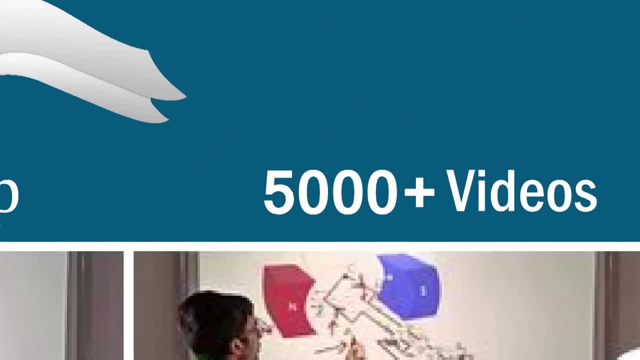 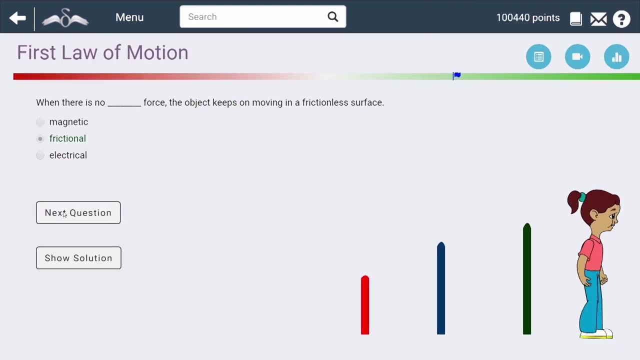 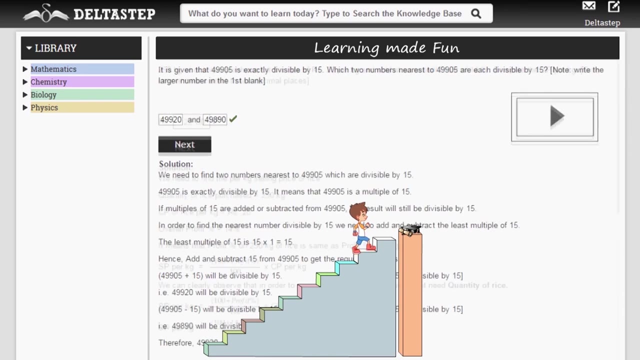 amazing teachers or to get access to all our 5000 plus amazing videos as per your school syllabus. Master each topic with our adaptive practice technology. Get million plus questions with step by step solutions and unlimited mock tests. Get all your doubts resolved instantly.